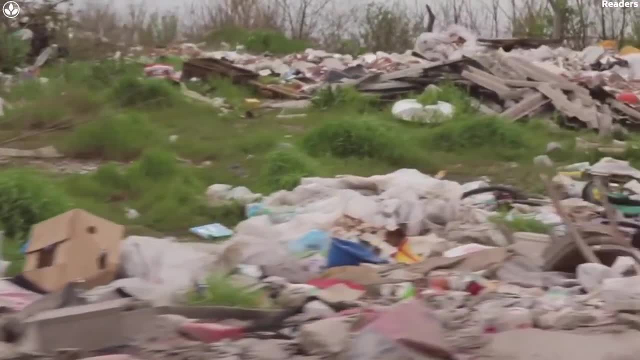 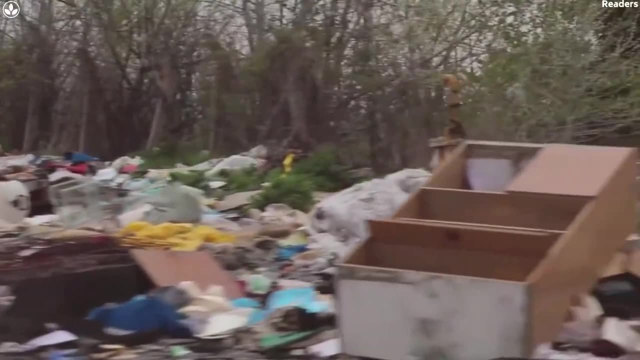 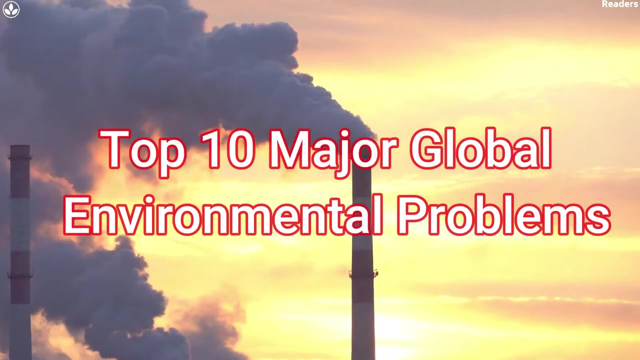 seem to be worsening with time, bringing us into a time of a true environmental crisis. It is therefore becoming increasingly important to raise awareness of the existence of these issues, as well as what can be done to reduce their negative impact. In this video, we have compiled the list of the top 10 main global environmental problems. 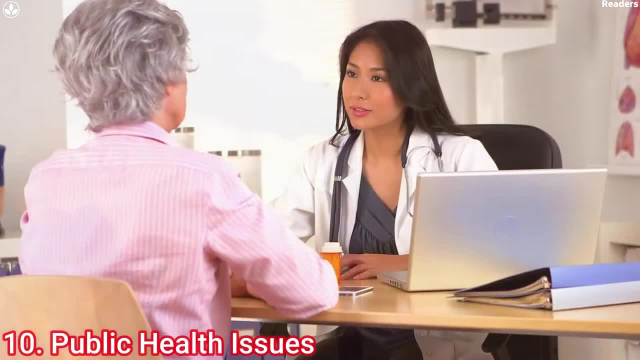 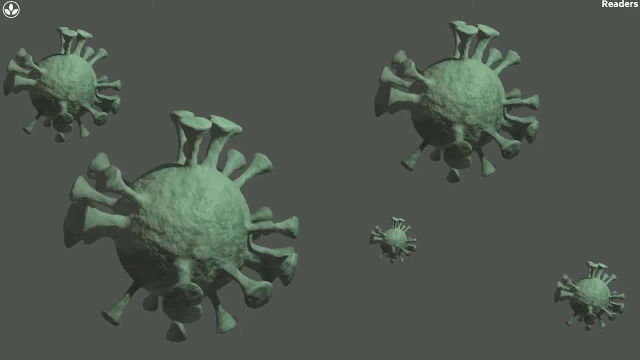 which the United Nations says we need to resolve. Number 10. Public Health Issues. There are various ethical dilemmas faced by the healthcare sectors, especially at times of pandemics and health emergencies. The current environmental problems pose a lot of risks to the health of humans and animals. 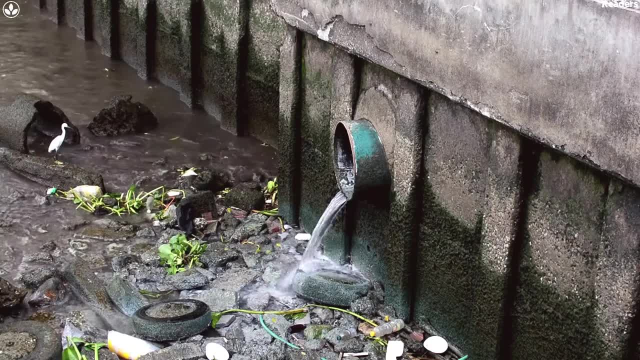 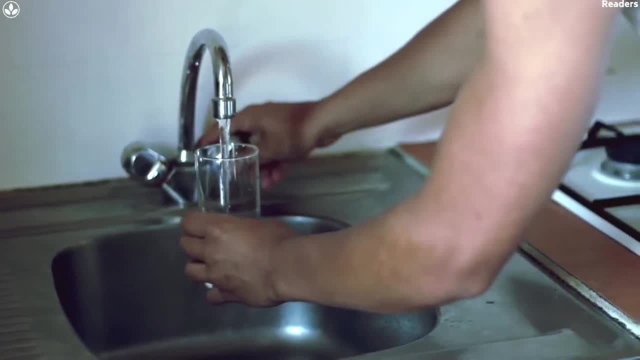 Dirty water is the biggest health risk in the world and poses a threat to the quality of life and public health. According to WorldCounts, every year nearly 1 million people die from water-related diseases, Most of them are children. Runoff to rivers carries with it toxins, chemicals. 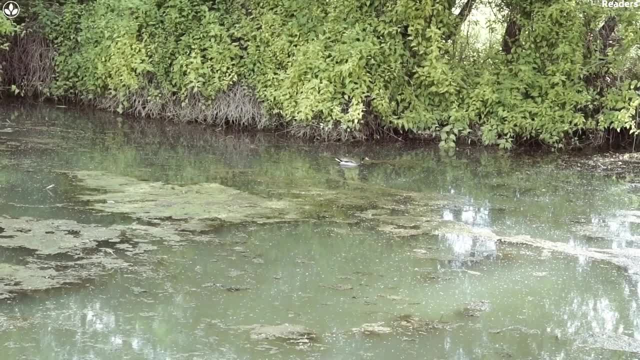 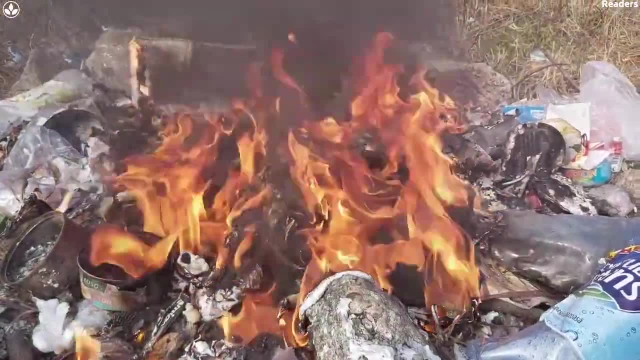 and disease-carrying organisms. Pollutants cause respiratory diseases like asthma and cardiac vascular problems. High temperatures encourage the spread of infectious diseases like dengue. There is a need for changes to be made in the public policies and health policies so that the 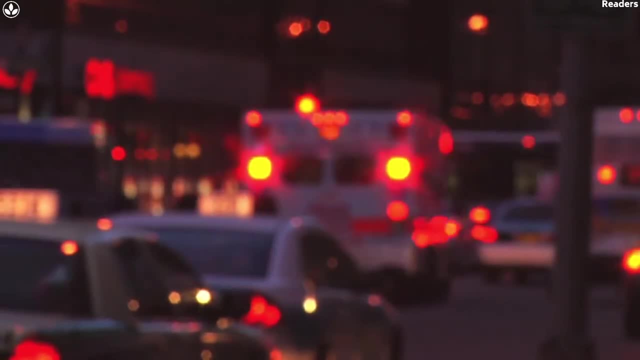 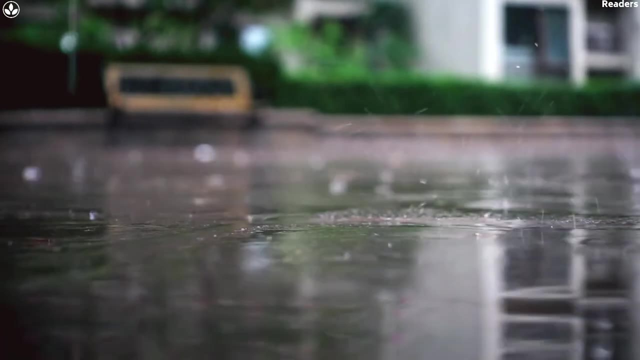 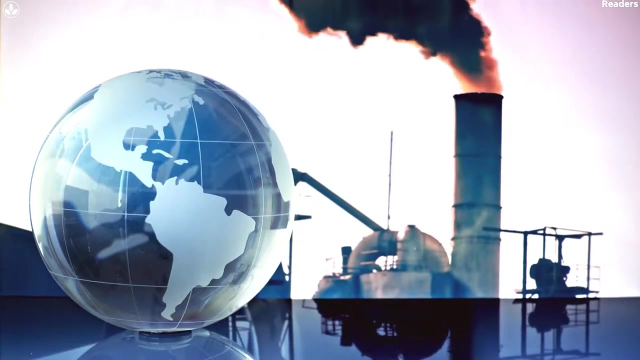 public health institutions are more prepared to deal with emergencies such as the one created by the Covid-19 pandemic Number 9.. Acid Rain: Acid rain occurs due to the presence of certain pollutants in the atmosphere. atmosphere Acid rain can be caused due to combustion of fossil fuels or erupting volcanoes or rotting. 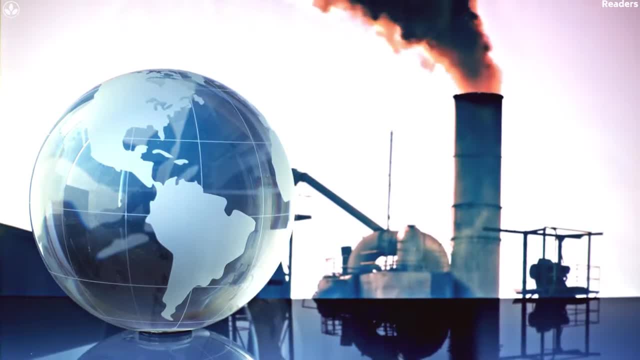 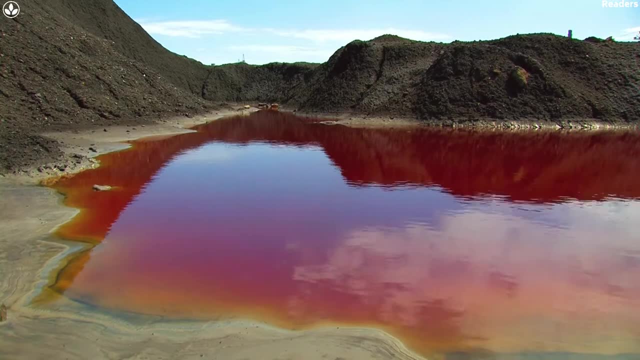 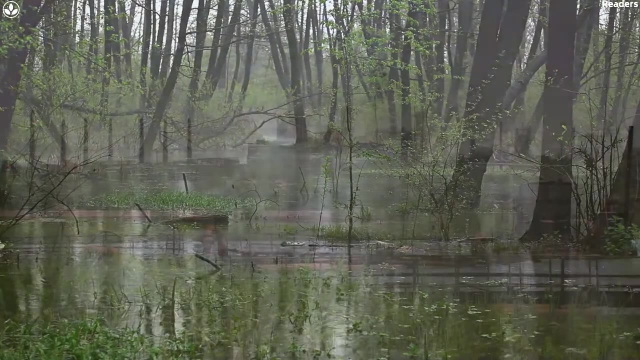 vegetation, which releases sulfur dioxide and nitrogen oxide into the atmosphere. Acid rain is a known environmental problem that can have a serious effect on human health, wildlife and aquatic species. Acid rain has also been shown to have adverse impacts on forests, freshwaters and soils. 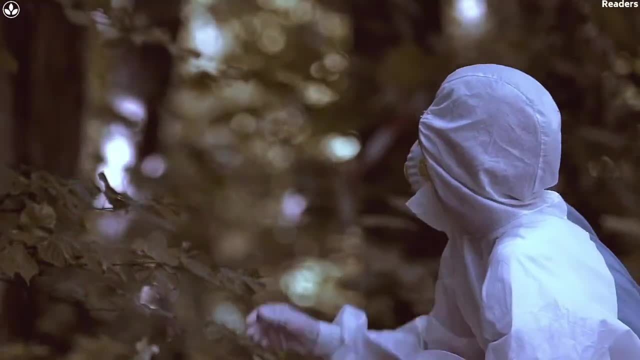 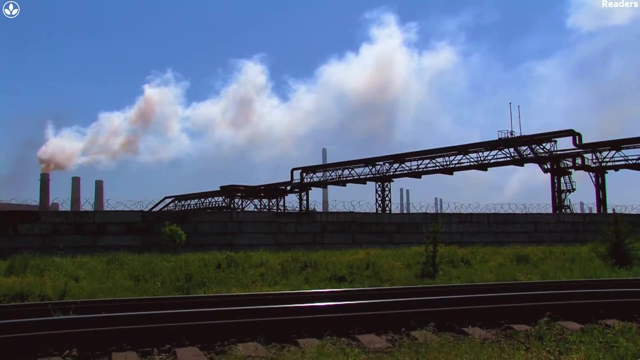 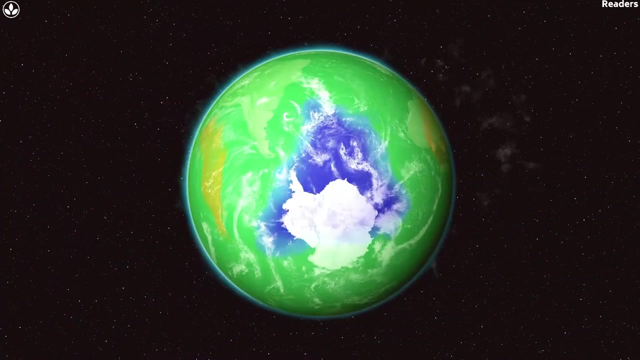 killing insect and aquatic life forms, causing the paint to peel, corrosion of steel structures such as bridges, and weathering of stone buildings and statues, as well as having impacts on human health. Number 8. Ozone Layer Depletion. The ozone layer is an invisible barrier of protection that wraps around the world, shielding 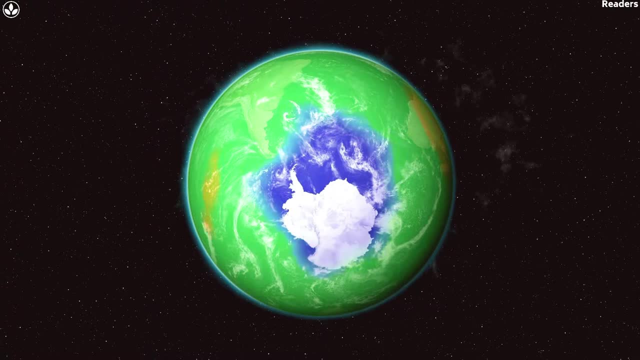 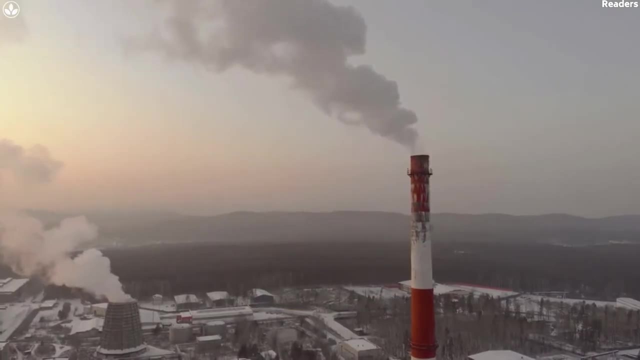 humans from the sun's damaging radiation. Pollution from chlorine and bromide, present in chlorofluorocarbons, is blamed for the depletion of the atmosphere's protective ozone layer. When these poisonous chemicals reach the high atmosphere, they cause a hole in the ozone. 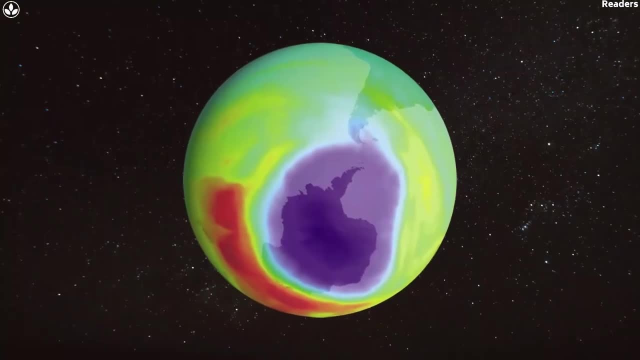 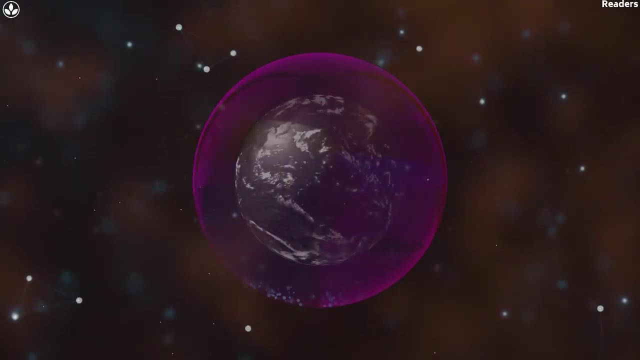 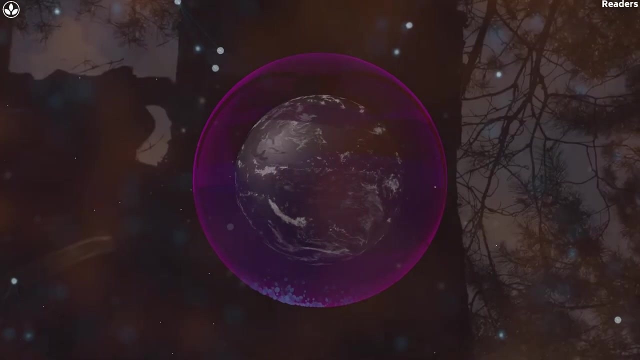 layer, the largest of which is located above Antarctica. CFC are prohibited in a wide range of businesses and consumer products. The ozone layer is valuable because it protects the world from damaging ultraviolet rays. This is one of the most serious environmental problems of the day. 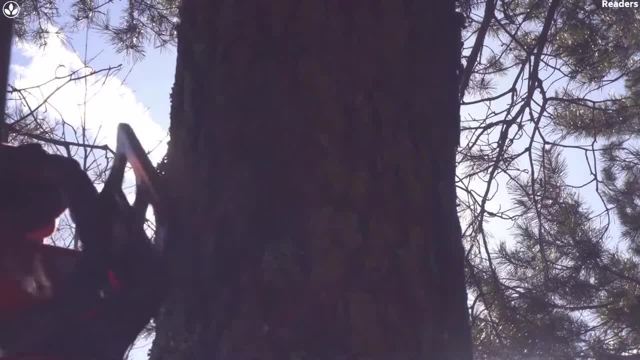 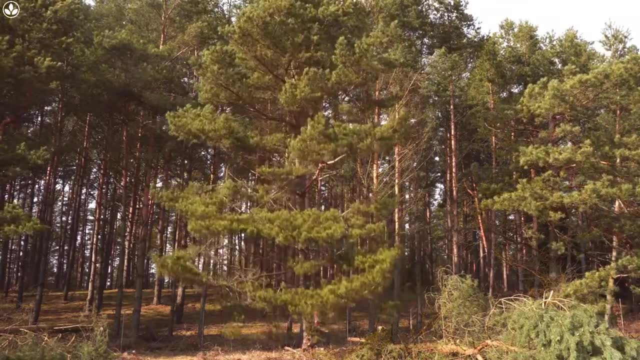 Number 7. Deforestation: Our forests are natural carbon dioxide sinks that also provide for the environment. They also provide fresh oxygen and aid in temperature and rainfall regulation. Currently, forests occupy 30% of the area, but every year tree cover is lost equating. 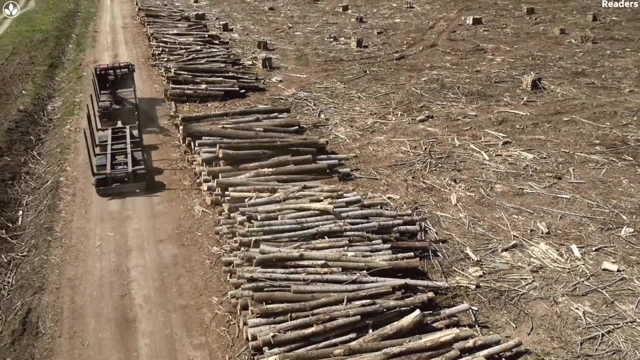 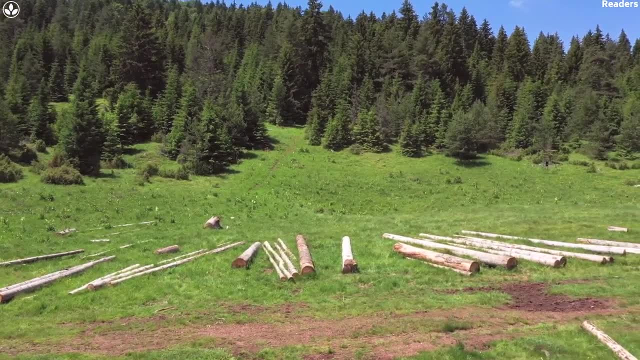 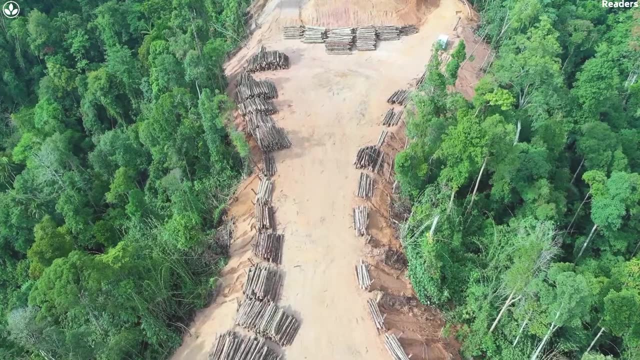 to the entire country of Panama due to the expanding population demand for more food, shelter and fabric. Deforestation simply refers to the removal of green cover in order to make land available for residential, industrial or commercial use. The surplus carbon is stored in the plant, helping it to grow. 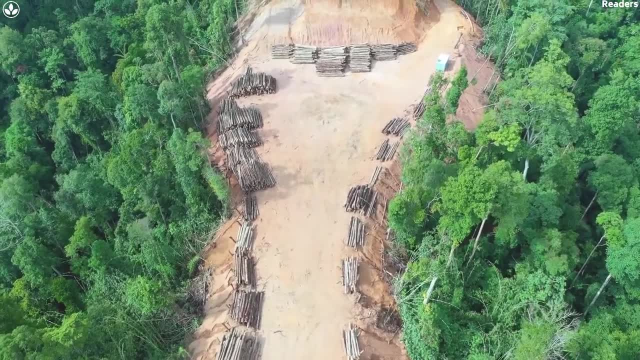 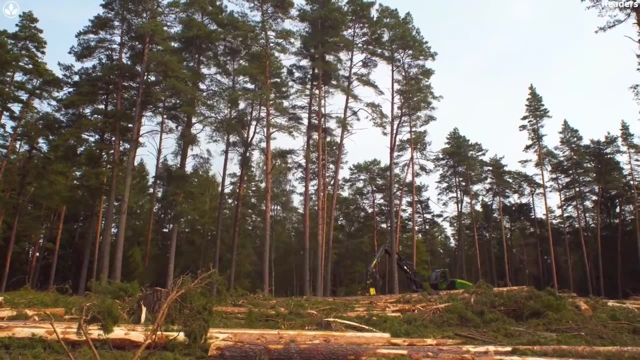 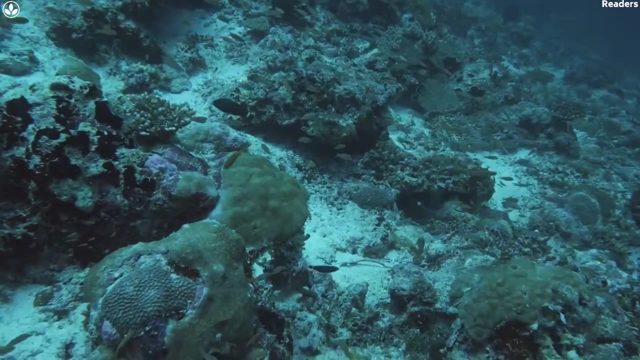 When trees are cut down and burned or allowed to rot, their stored carbon is released into the air as carbon dioxide, And this is how deforestation and forest degradation contribute to global warming. Number 6. Loss of Biodiversity: Human activity is causing the extinction of species and habitats, as well as the loss 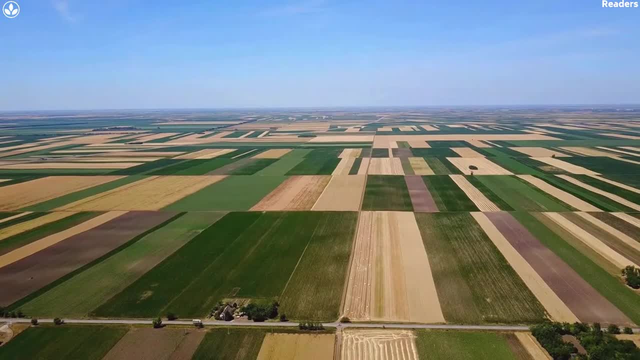 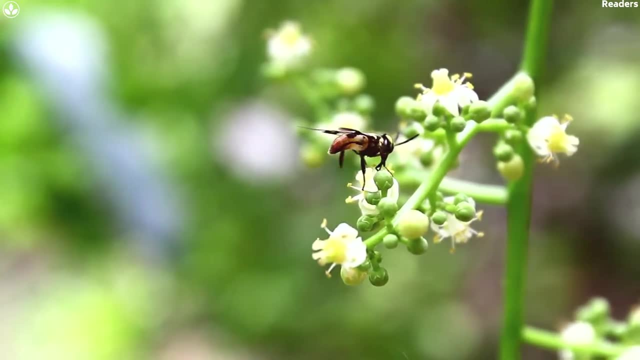 of biodiversity. Ecosystems that have taken millions of years to perfect are in trouble. when any species population is decimated, The balance of the number of species is so small that it is based on the population. What are the causes? natural processes such as pollination is critical to the existence of the ecosystem. 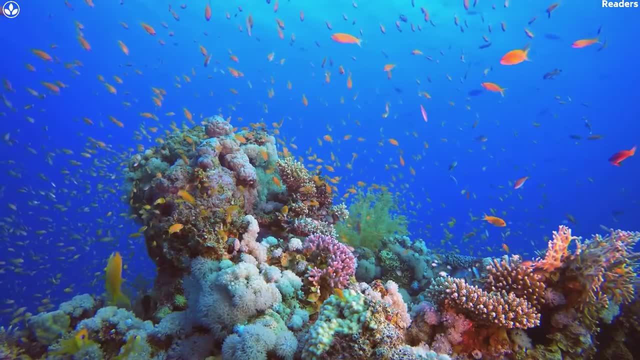 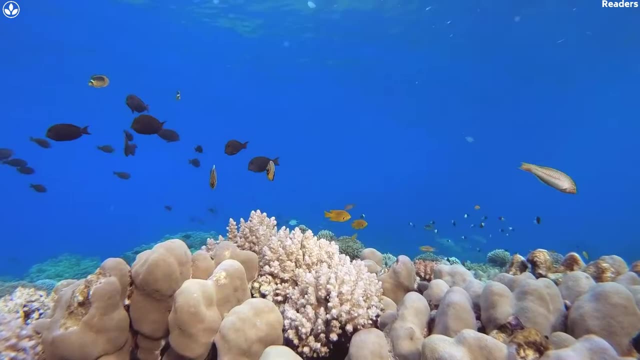 and human activity threatens it. Another example is the destruction of coral reefs in the world's oceans, which support a diverse range of marine life. Biodiversity loss can have significant direct human health impacts if ecosystem services are no longer adequate to meet social needs. 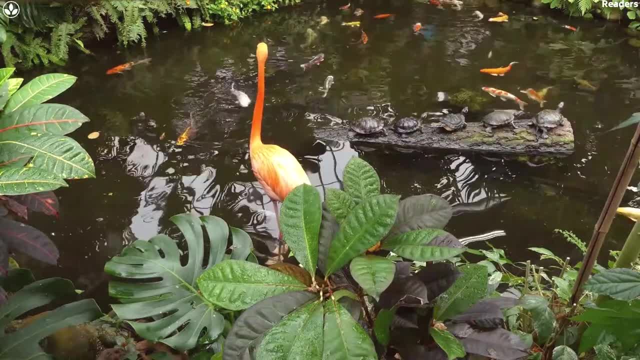 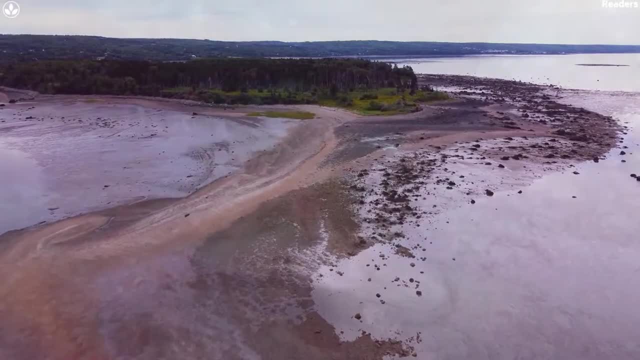 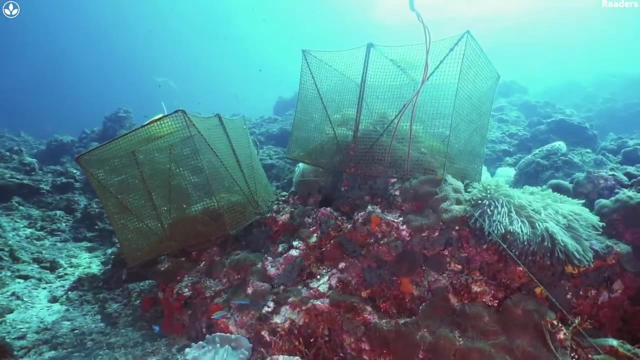 Indirectly. changes in ecosystem services affect livelihoods, income, local migration and, on occasion, may even cause or exacerbate political conflict. Number 5. Ocean Acidification. Ocean acidification is the ongoing decrease in the pH value of the Earth's oceans caused by the uptake of carbon dioxide from the atmosphere. The main cause of ocean acidification is the burning of fossil fuels. Ocean acidification is one of several effects of climate change on oceans. Ocean acidity has increased by the last 250 years. Ocean acidification is one of several effects of climate change on oceans. 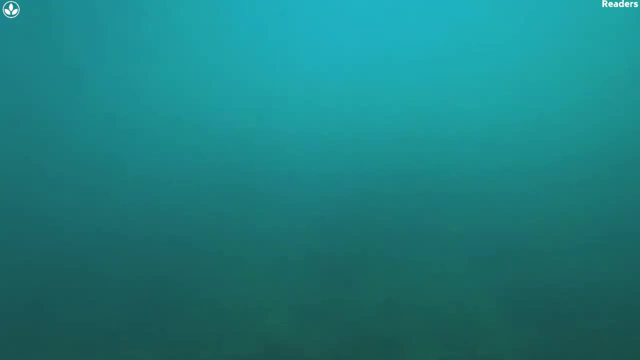 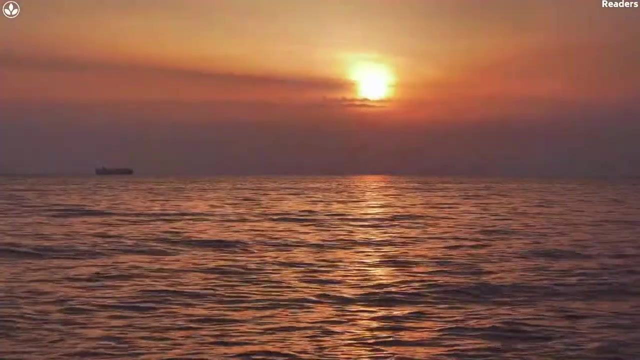 Ocean acidification is two-thirds of the total amount of carbon dioxide emitted by ocean acidification today, but by 2100, it may shoot up by 150%. The main impact is on shellfish and plankton, in the same way as human osteoporosis. Ocean acidification can also modify the abundance. 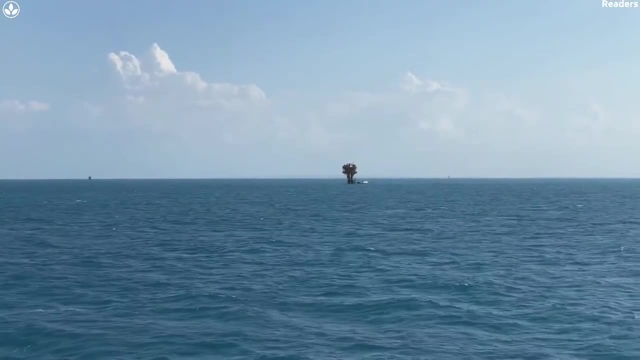 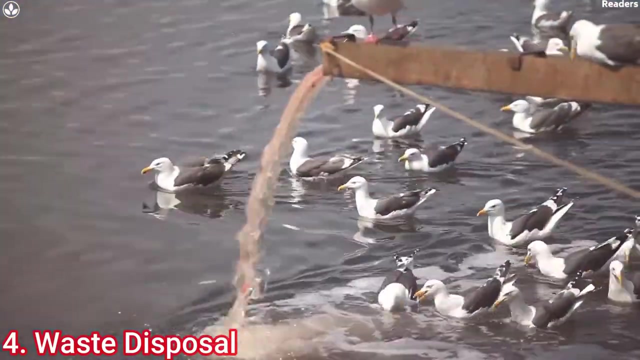 and chemical composition of harmful algal blooms in such a way that shellfish toxicity increases and therefore human health is negatively affected. Number 4. Waste Disposal. Waste disposal has significant environmental consequences and can lead to catastrophic environmental consequences. This can be a 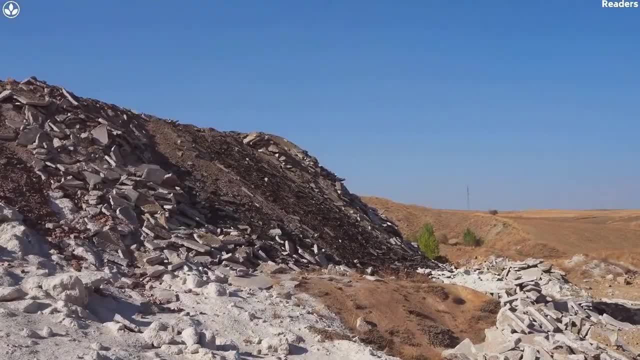 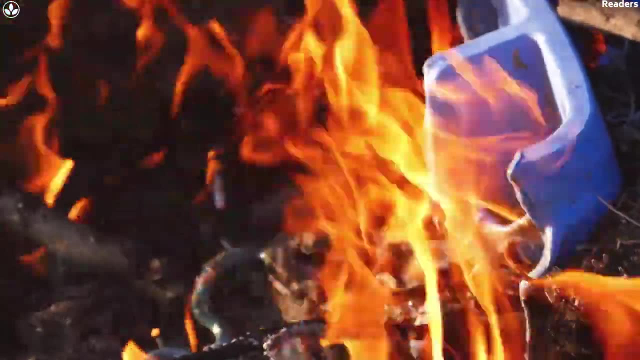 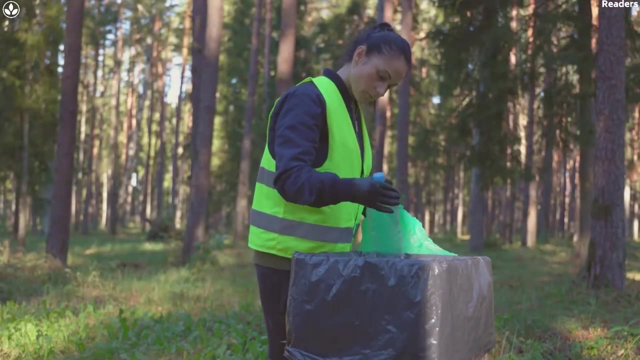 to catastrophic difficulties. Overconsumption of resources and the production of plastics are causing a global waste disposal dilemma. Developed countries are infamous for producing an excessive amount of waste or junk and dumping it in the oceans, while less developed countries are notorious for producing an insufficient amount of waste or garbage. The disposal of nuclear waste. 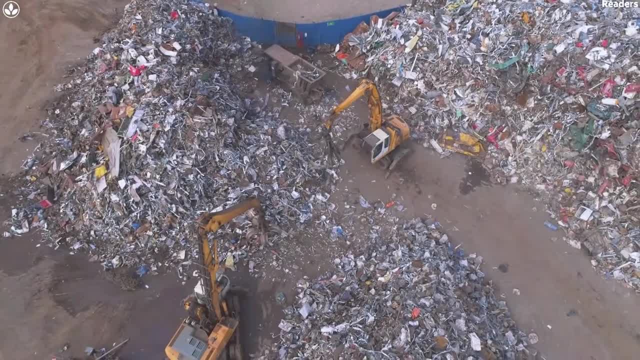 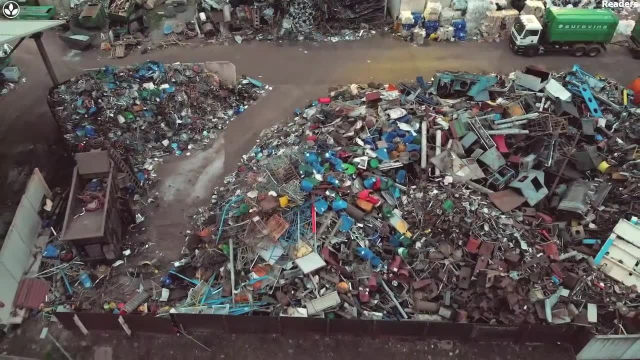 poses significant health risks. Plastic fast food packaging and low-cost electronic waste endanger human health. Some garbage will ultimately decay, but not all, and in the process it may smell or produce explosive methane gas, which contributes to the greenhouse effect. 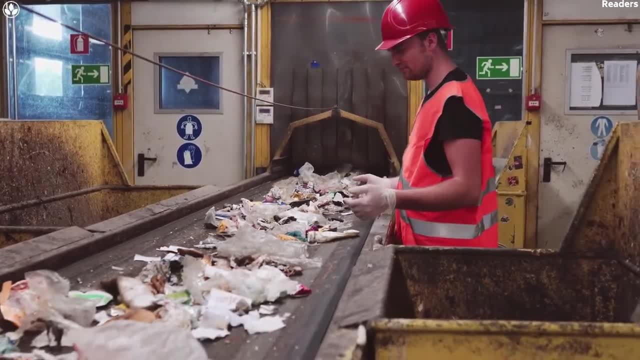 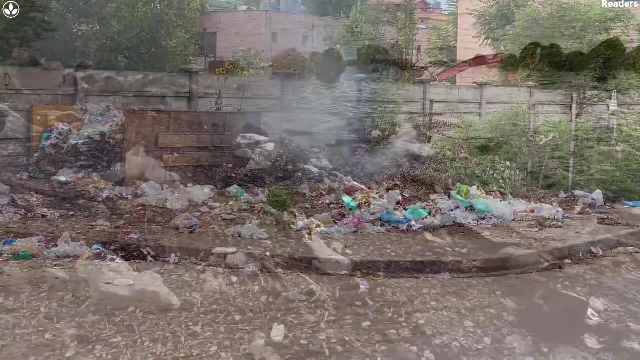 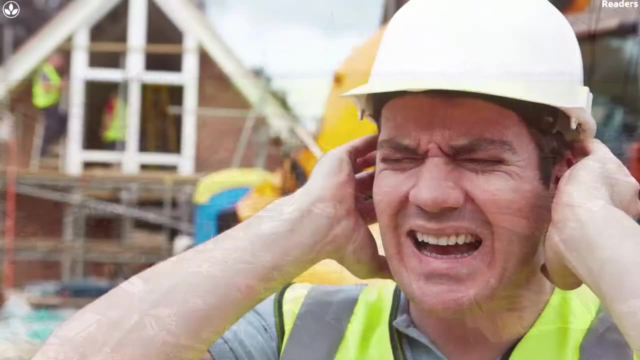 Leachate formed as garbage decomposes has the potential to pollute the environment. As a result, waste disposal is one of the most serious current environmental issues. Number 3. Pollution. There are seven major categories of pollution: Air, water, soil, noise. 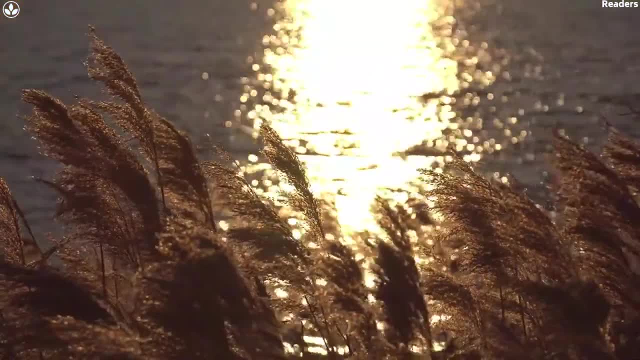 radioactive and pollution. There are seven major categories of pollution. There are active light and thermal, and they are the principal reasons that have a wide range of effects on our environment. All of these types of pollution are interconnected and have an impact. 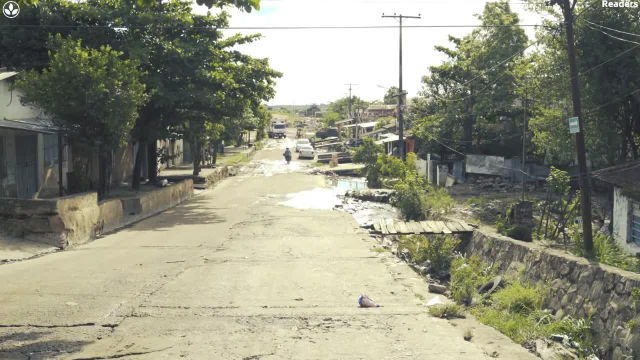 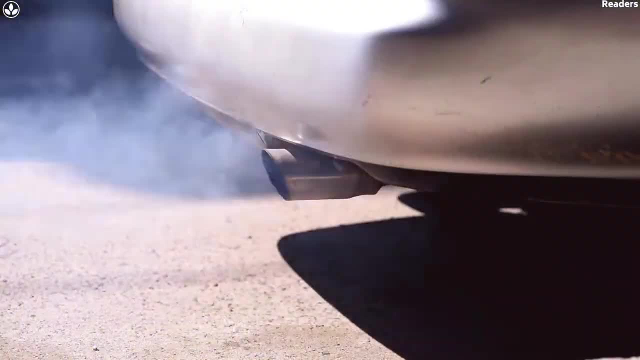 on one another. Therefore, we need to tackle all of them together. Pollution of the air, water and soil takes millions of years to recover from. The most significant pollutants are those emitted by industry and motor vehicles. Toxins that cause pollution include heavy metals. 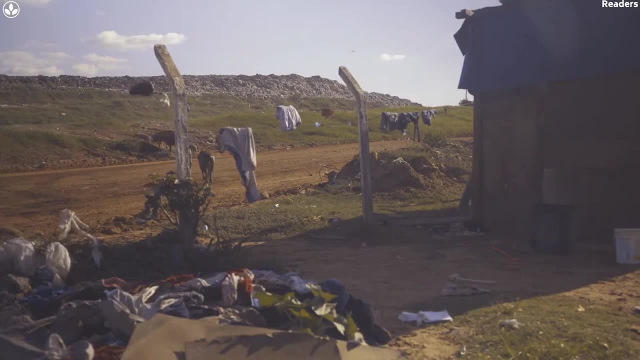 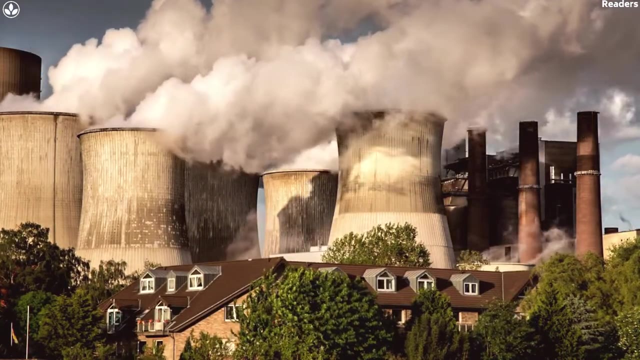 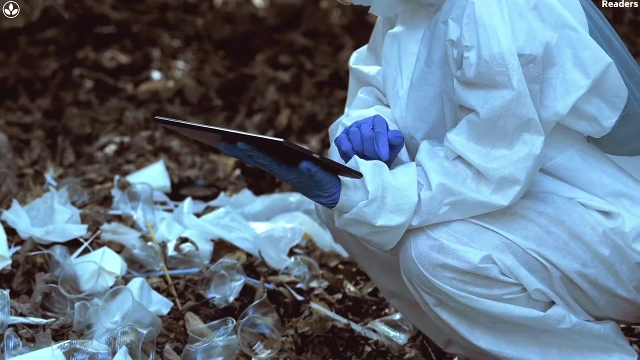 nitrates and plastic. While oil spills, acid rain and urban runoff cause water pollution, air pollution is caused by various gases and toxins released by industries and factories, as well as the combustion of fossil fuels. Soil pollution is primarily caused by industrial waste, which deprives soil of essential nutrients. 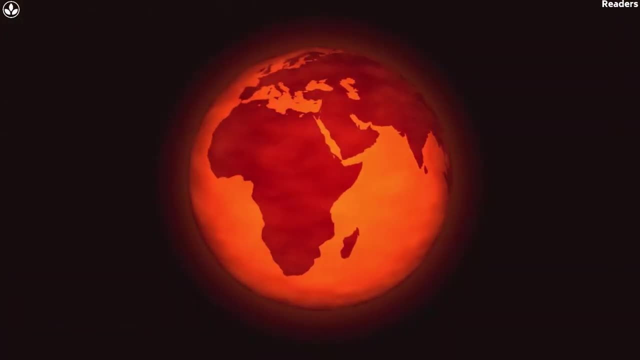 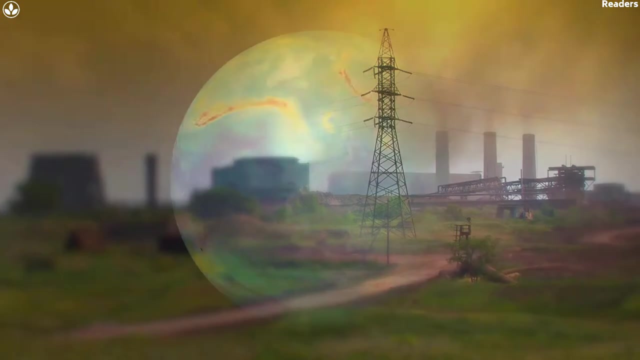 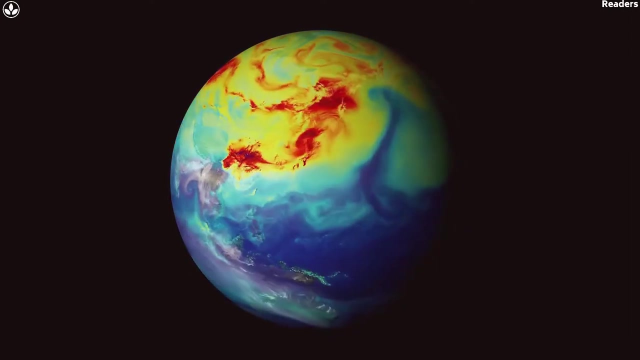 Number 2. Global Warming. Since the Industrial Revolution, the global annual temperature has increased in total by a little more than 1 degree Celsius. Between 1,800 and 1,000,000 people live in the world. Since 1980,, the year that accurate record-keeping began, and 1980, it rose on average by 0.07 degrees.